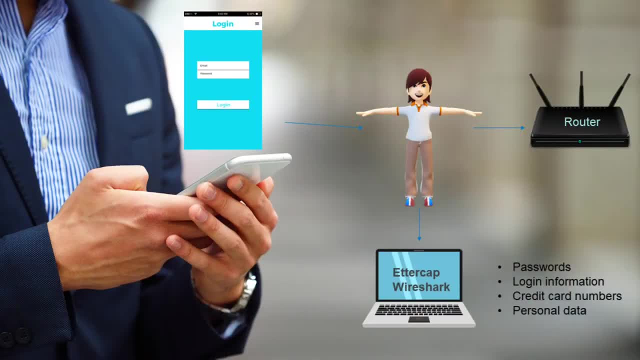 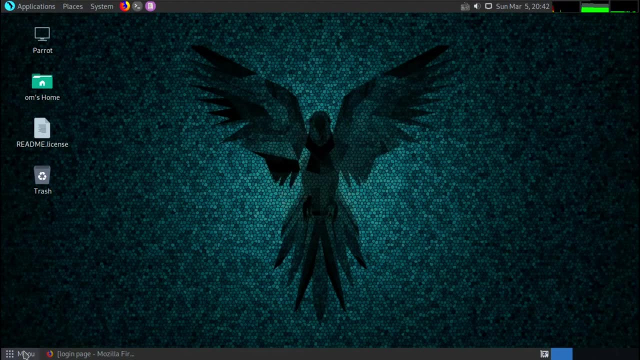 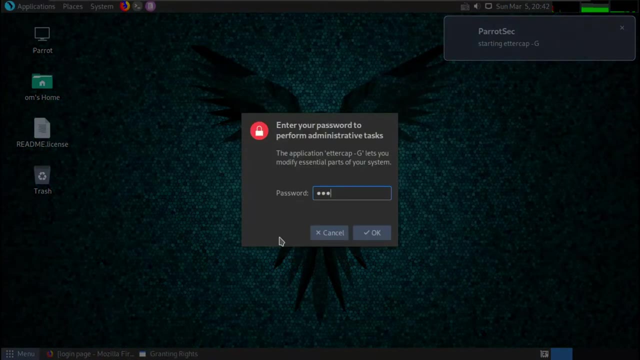 of emails or messages, redirecting web traffic to malicious websites or even injecting malware into the victim's device. Let's see practically. here I am going to use tool called ethercap, which is already available on my parrot os dot. let's open. 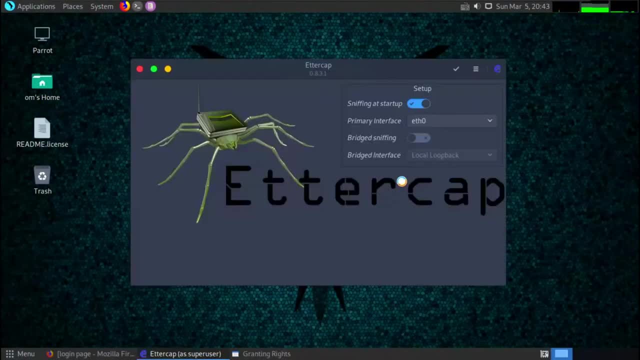 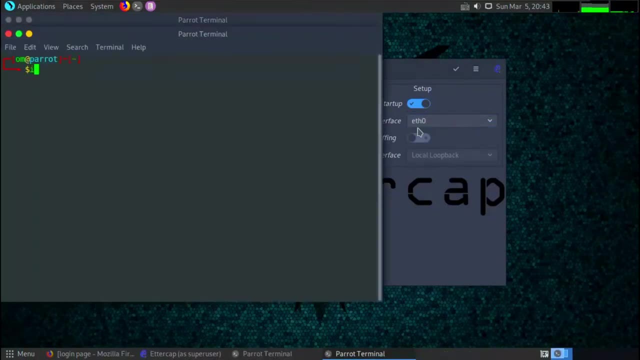 It's asking me for password. Let's give the password. Now, here we have to select interface, which is I am going to do with my Wi-Fi. So my interface name is ethernet zero. You can see the interface name from your ifconfig command. 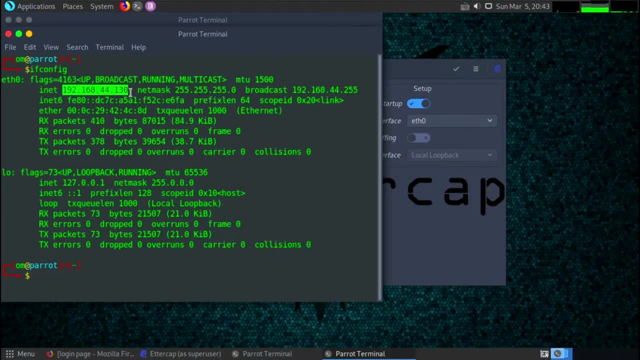 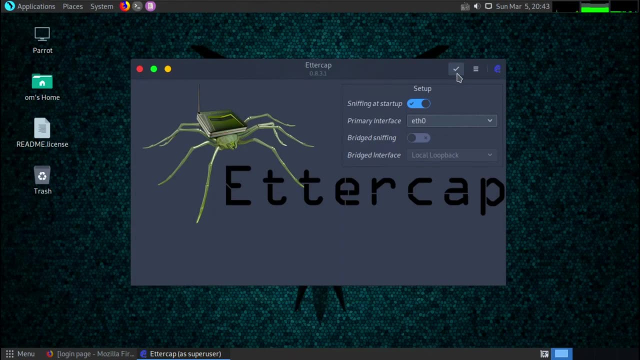 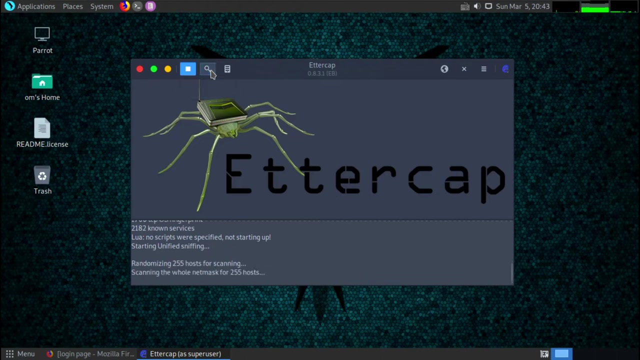 Here. My laptop IP address is one nine two dot one, six eight dot four four dot one, three zero. Okay, so let's start. click on this right sign. tick. Now we are in listening mode. We need to search for the host first, So just click on this search button over here. 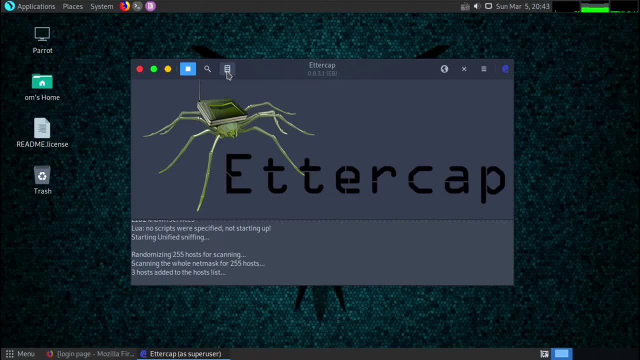 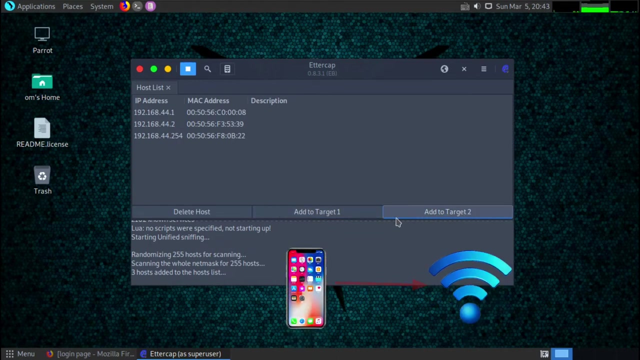 Here we can see three host added to the host list. Okay, so let's see the host list by clicking this host list icon And here in this host list we have to select to target host. Target one will be your mobile phone and the target two will be your router. 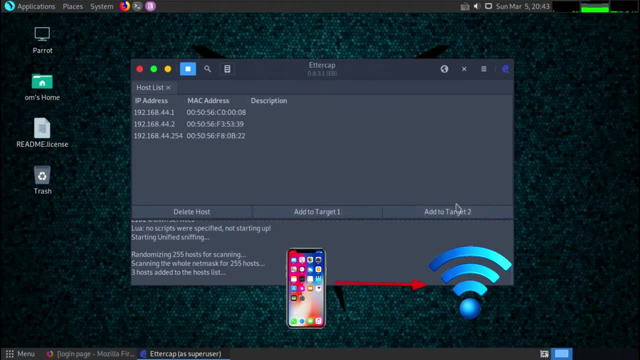 Because here all the traffic is going from your mobile phone to router And we are intercepting this packets. So we also should not know the IP address of mobile phone. But here we don't need the actual IP address or MAC address of the mobile phone. 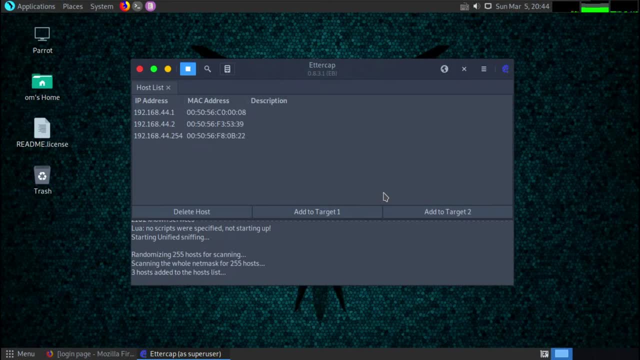 We need the MAC or IP provided by the DHCP server from the router So we can identify the devices. Go to your phone's connected WiFi setting and see the IP address which is assigned by router. In my case, my phone's IP address is one nine, two dot one, six, eight dot four, four dot two. 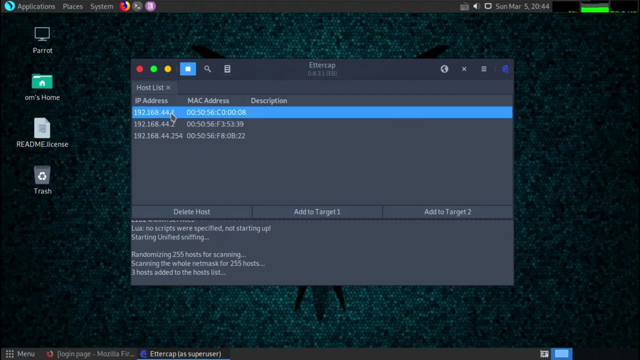 And the IP one, nine, two dot one, six, eight, dot four, four dot one is the IP address of my router. So let's select phone's IP as target one and the router, which is by default point one. So I will select it as target two. 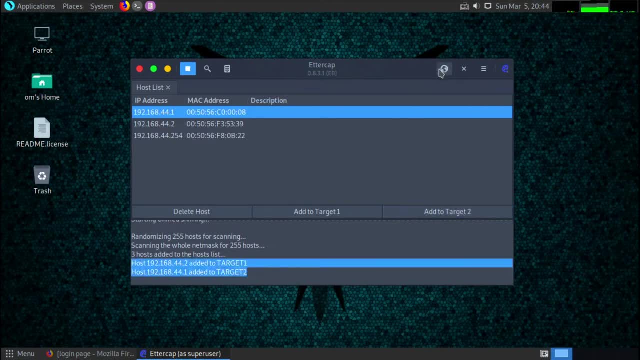 Okay, so both the target are selected. Now go in this MITM menu, which is man in the middle attack. Now we have to select the type of attack. In many normal attack there are lots of type of attack. Here I am going to use ARP poisoning. 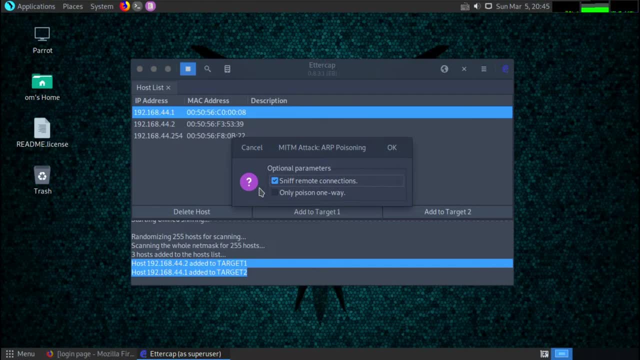 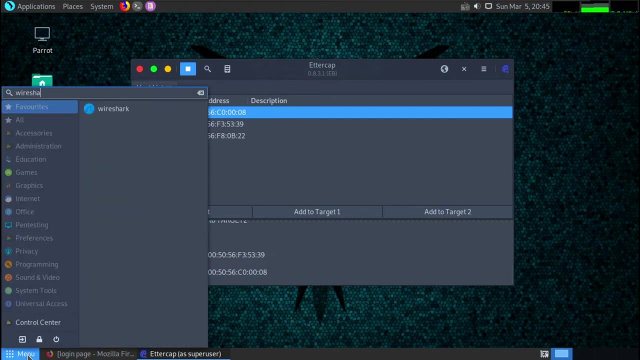 So just select ARP poisoning And here click on ARP poisoning, Click on sniff remote connection and click on okay, The attack is launched. now We can actually see what my mobile phone or victim device is doing with internet And we can actually see if the user is passing any login credential. then we can get that. 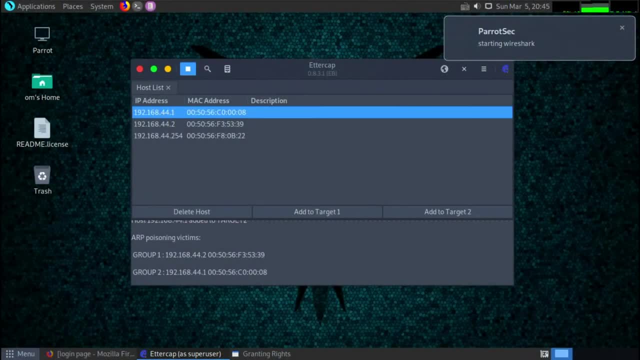 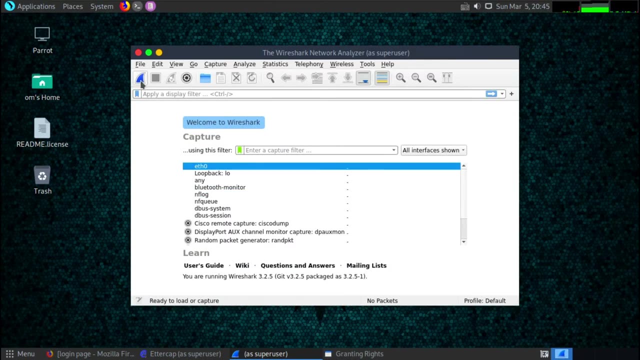 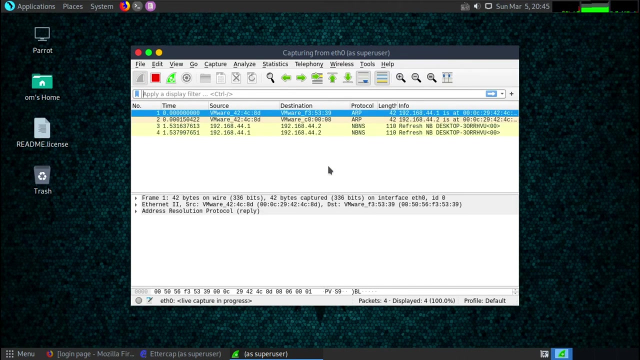 login credential How I am going to show you We are going to snap the packet in the network with the help of tool called Wireshark, Asking for the password. I will simply start the Wireshark from here and my Wireshark keeps sniffing all the packets in the network. 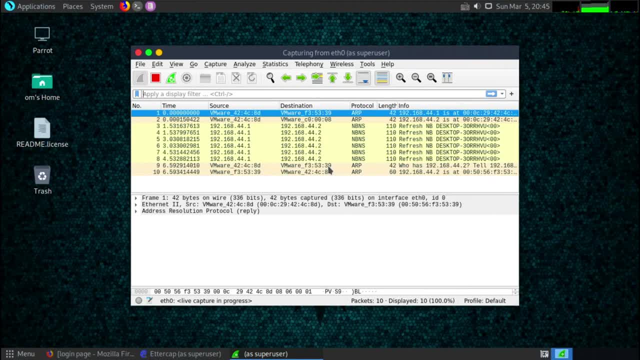 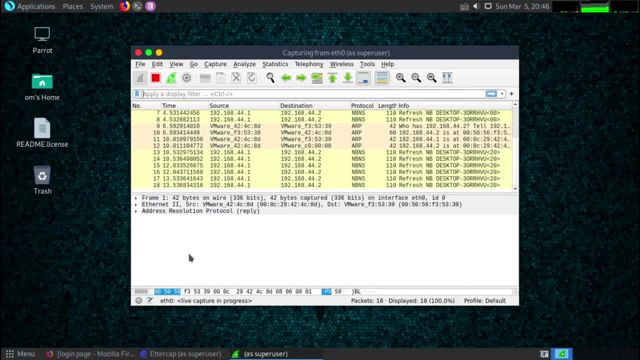 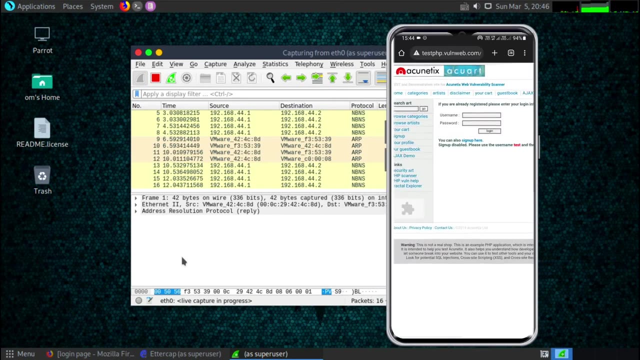 Okay, so we are in middle of my mobile phone and router, So we can actually see what's my mobile phone and router is communicating. Okay, so what I will do? I will show this small demonstration with my Google Chrome. I will open one demo side which is not secure by HTTPS program. 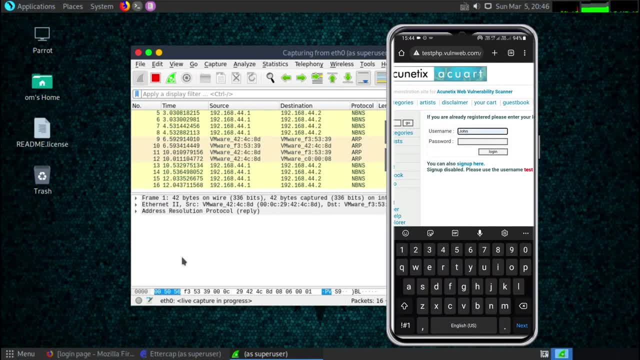 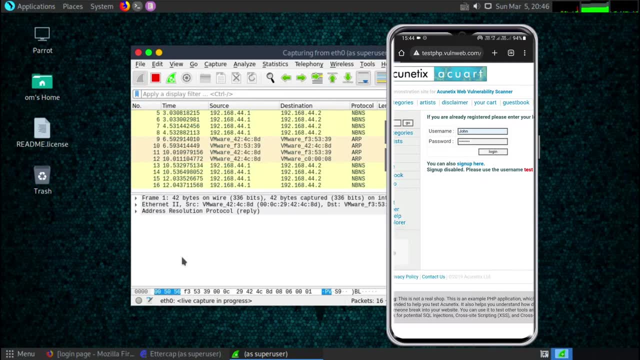 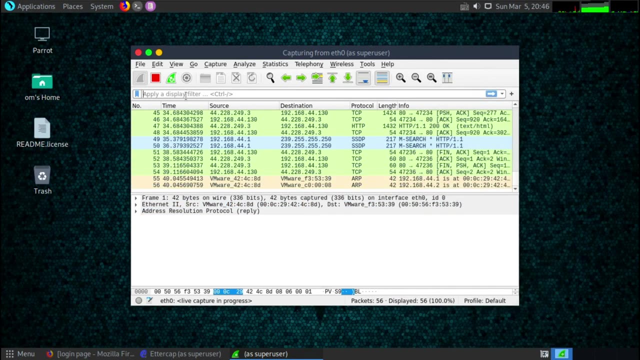 protocol here. i am going to give the username as john and password as john at one to three. just click on login. the credentials are wrong so i didn't get logged into it, but the credential has been captured by our packet tracer, which is wireshark. because we are in middle of my phone. 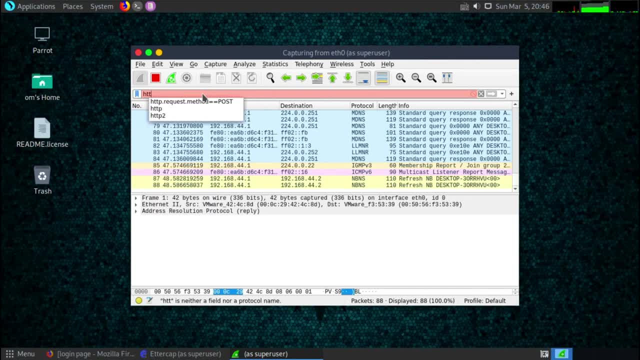 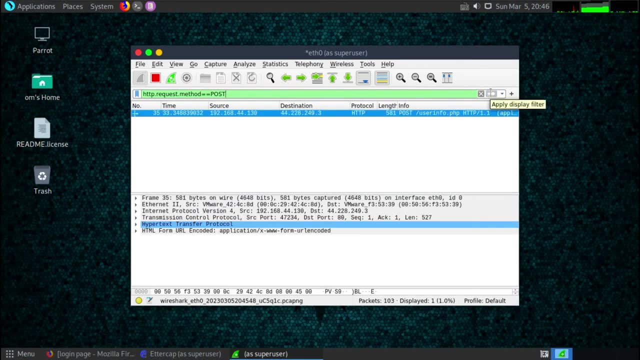 and router. okay, so how you can see that? just, you have to go for http site, then type this query to see only http packets: http dot r. equest method is equal to is equal to post and hit enter. here you can see one packet has been captured from the http site. so let's see what data this packet has. 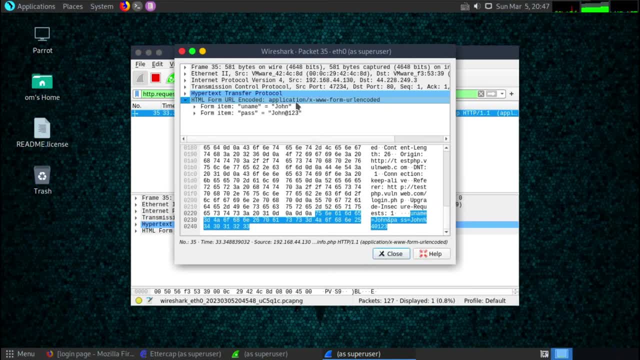 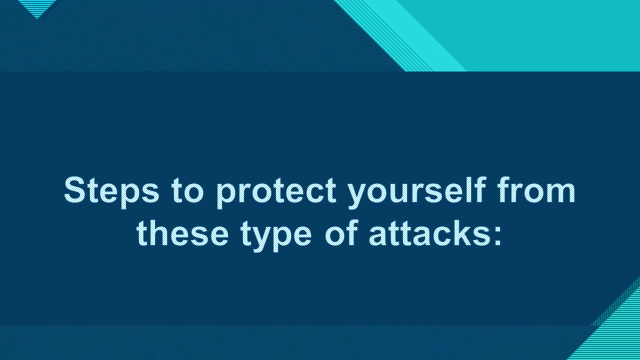 captured. okay, so just go into html form url encoded in that section. you can see the username and password here. username is john and password as john at one to three. in this way, your credential can be stolen if you are using an public or open wi-fi. here are some steps you can take to protect yourself from these type of attacks. use a secure. 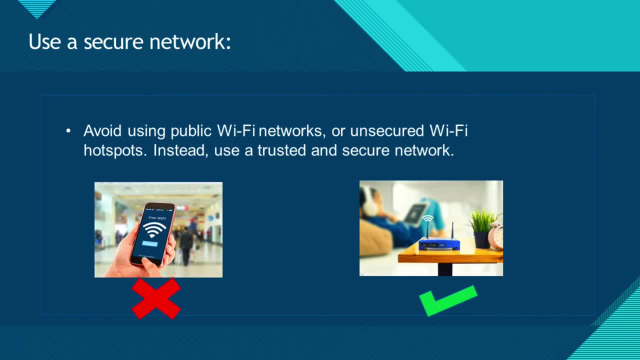 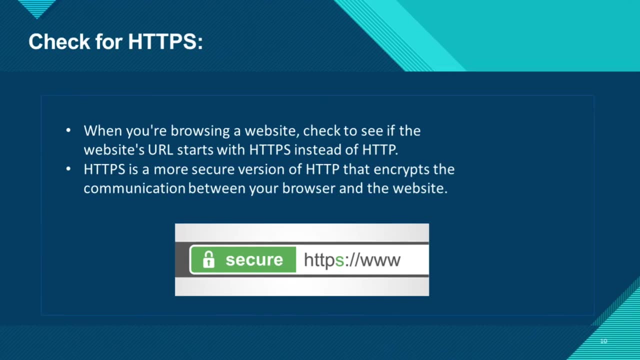 network. avoid using public wi-fi networks or unsecured wi-fi hotspots. you can see the username and password here. username is john and password as john at one to three. instead, use a trusted and secure network. check for https when you are browsing a website. check to see if the website's url starts with https instead of http. https is a more secure 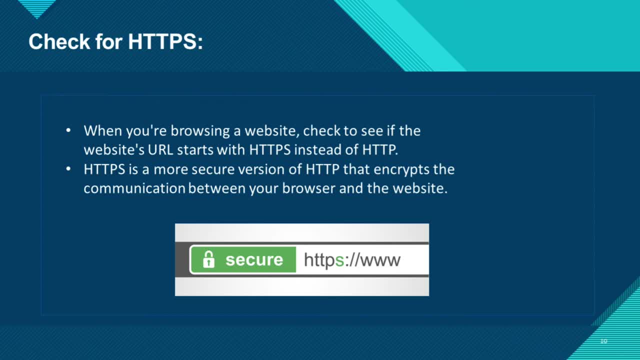 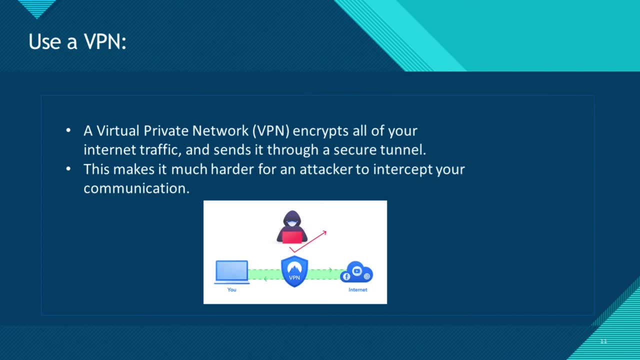 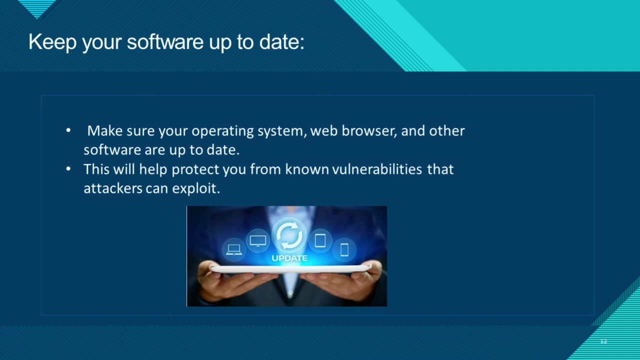 version of http that encrypts the communication between your browser and the website. use a vpn, a virtual private network. vpn encrypts all of your internet traffic and sends it through a secure tunnel. this makes it much harder for an attacker to intercept your communication. keep your software up to date. make sure your operating system, web browser and other 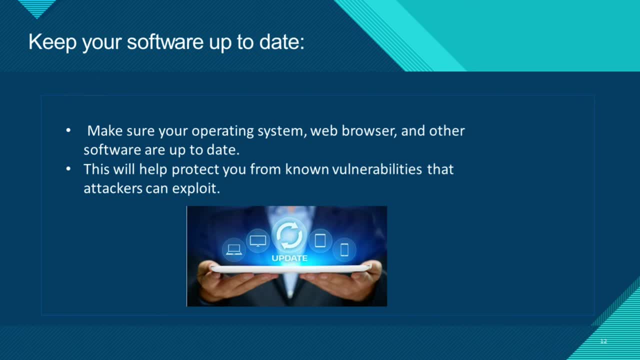 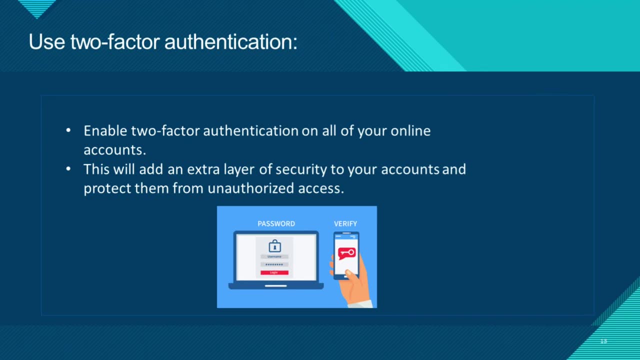 software are up to date. this will help protect you from known vulnerabilities that attackers can exploit. use to factor authentication. enable to factor authentication on all of your online accounts. this will add an extra layer of security to your accounts and protect them from unauthorized access. be cautious of suspicious links. be careful when clicking on links that you receive in emails. 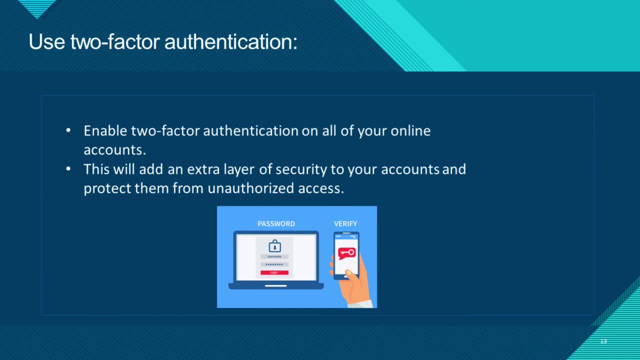 or messages, scammers may try to trick you into clicking on a link that leads to a malicious website or installs malware on your device. by taking these steps, you can reduce the risk of falling victim to man-in-the-middle attacks and attacks and attacks on your device. you can also.